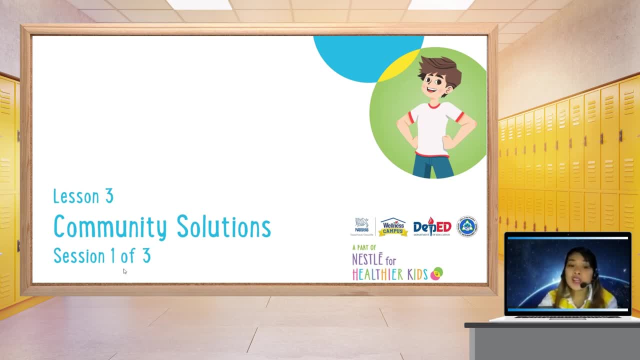 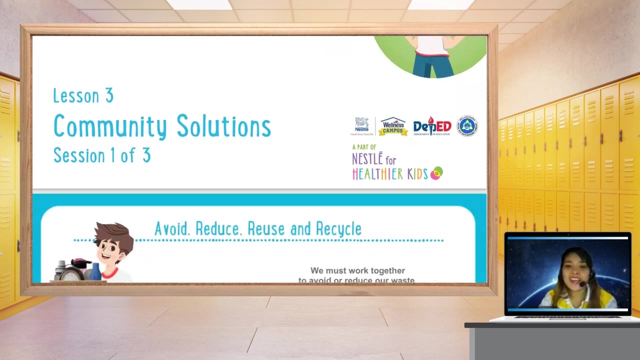 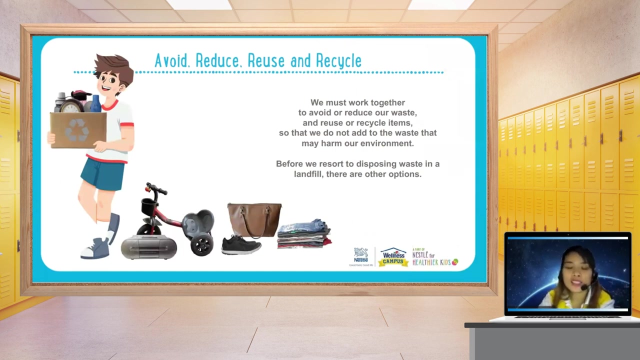 learn on how we can find solutions, all right, in our community. All right, So are you ready for this? All right, So what are we waiting for? Let's start. Okay, So last time we were able to talk about- right, with other lectures, right, the problems in our community. So what? 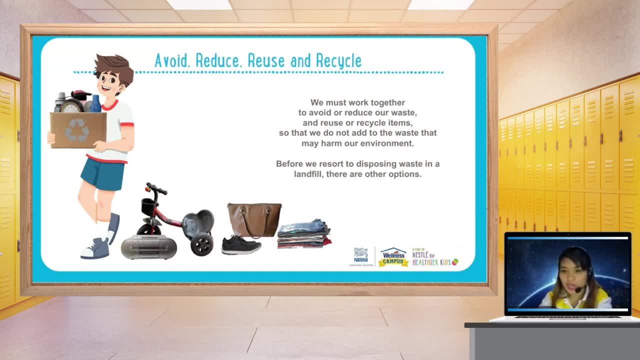 do we need to do? We should avoid, right. So we should reduce, reuse and recycle. So we must work together to avoid or reduce our waste and reuse or recycle items Just like what you know, what we have here in the picture, right. So before we resort to disposing waste in our 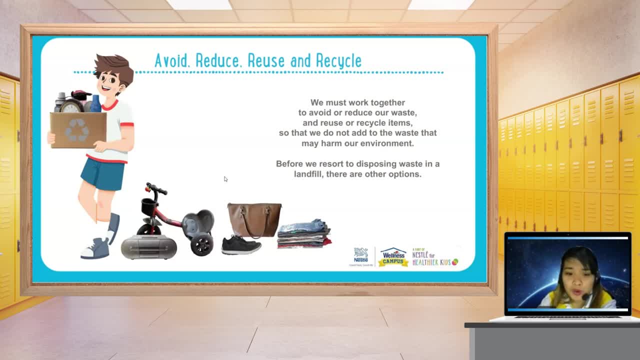 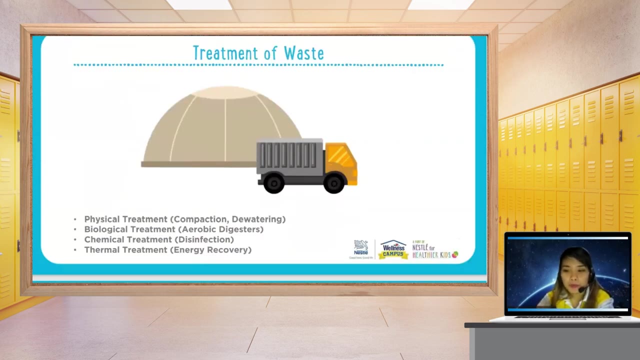 landfill. there are other options, right? So before you throw away that bike, someone might need it. Before you throw away that better bag, you can give it to a friend who needs one, okay, Okay. So, before we go on further, let's recall how do we treat waste, right? So the 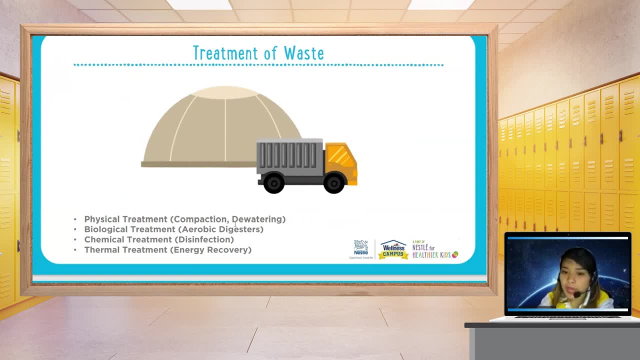 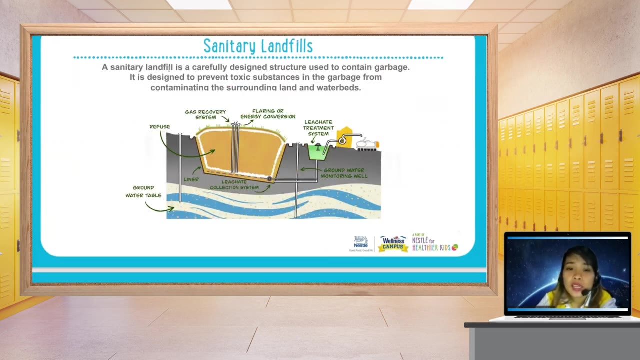 treatment of waste goes on like this: The physical treatment- compacting, watering right, Biological treatment, aerobic digesters- And the chemical treatment is disinfection. Thermal treatment is energy recovery. So a sanitary landfill is a carefully designed, structured use to contain garbage. It is designed to prevent toxic substances in the garbage from. 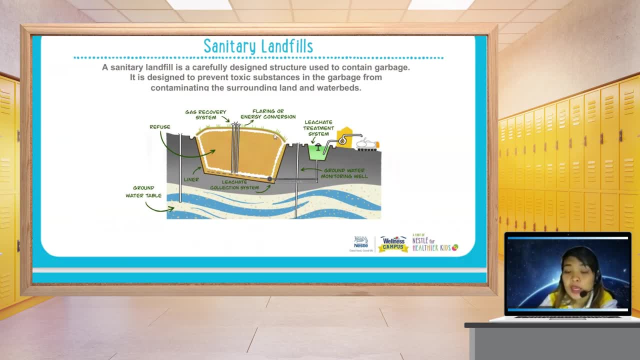 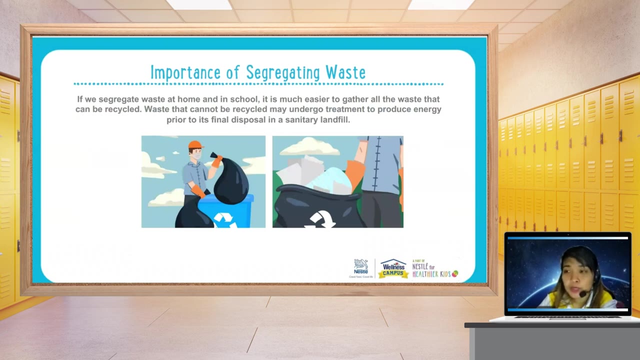 contaminating the surrounding land and waterbed. So how did they do that? They tried to dig on the ground right So that they put the waste in this big hole. So what is the importance of segregating waste? We all know that. We've been, you know. 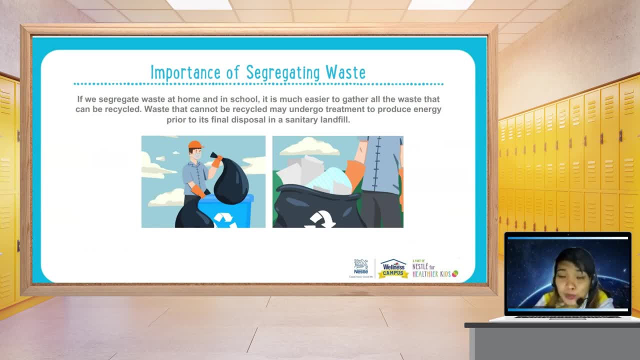 we've been teaching this for quite some time since you were in elementary right. So we've been teaching this for quite some time since you were in elementary right. So what is the importance of segregating waste? We all know that. We've been, you know. 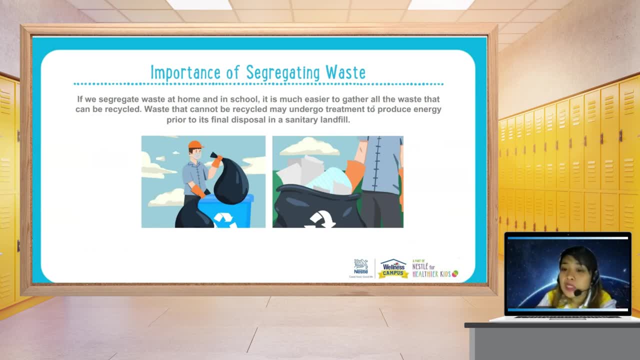 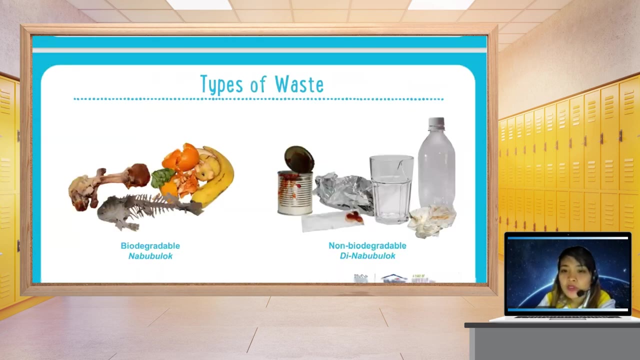 right. So if we segregate waste at home and in school, it is much easier to gather all the waste that can be recycled. So waste that cannot be recycled may undergo treatment to produce energy prior to its final disposal in a sanitary landfill. So what are the different types of waste? to begin, 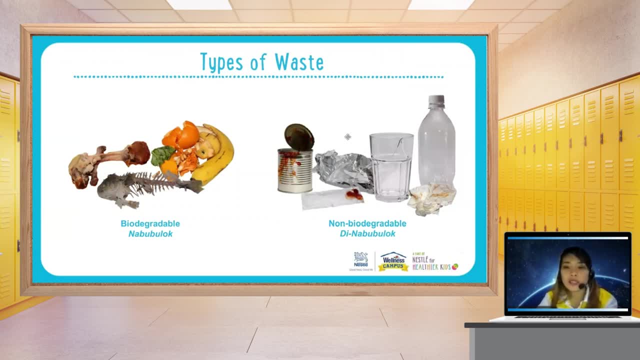 with right. So we have two right: The biodegradable, or in Tagalog it's nabubuyok right, And the non-biodegradable waste right. So we have two right: The biodegradable, or in Tagalog it's nabubuyok. 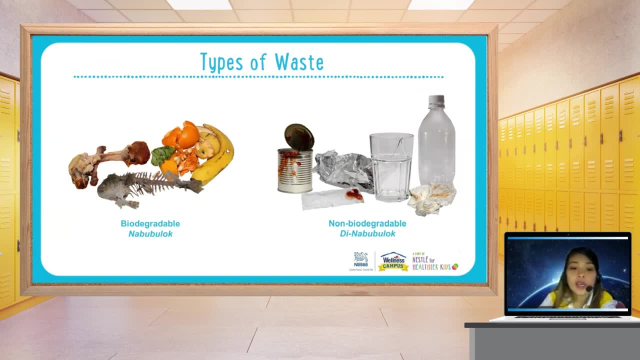 this is what we call in Tagalog as dinabubuyok. all right, So, as you can see here what are examples based on the picture? like the food waste, you know, like here fish right And the chicken bones right, The peelings of the banana, and then we have here tomato. 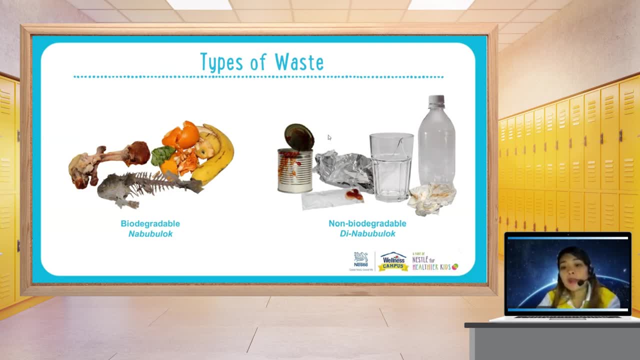 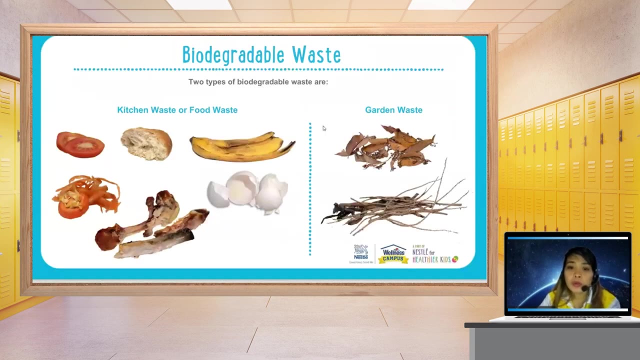 you know, these are examples of biodegradable And the non-biodegradable cans, right, like wrappers, bottles, plastic bottle, right, Those are examples of non-biodegradable, or in Tagalog as dinabubuyok. okay, So the biodegradable waste. there are two types of biodegradable waste. 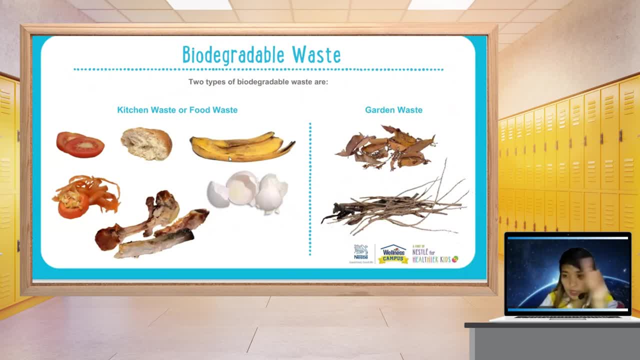 by the way, the kitchen waste or waste food, just like you know the example that we have earlier on- and the garden waste. you know we are talking about the leaves. you know falling out of the trees and the twigs from the trees. you know the leaves. you know the leaves. you know the leaves. 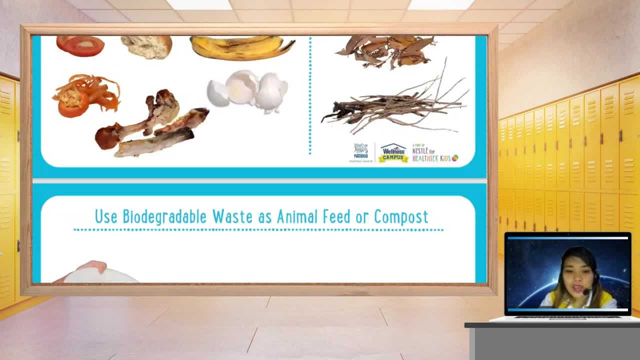 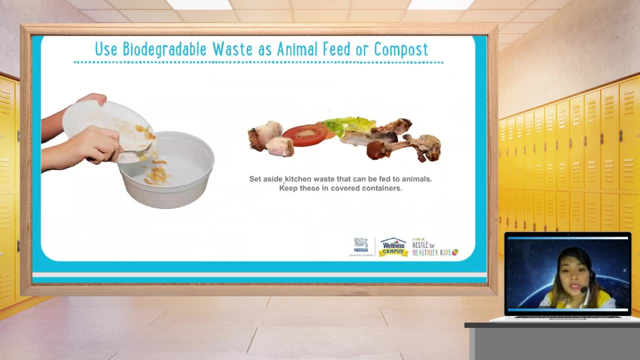 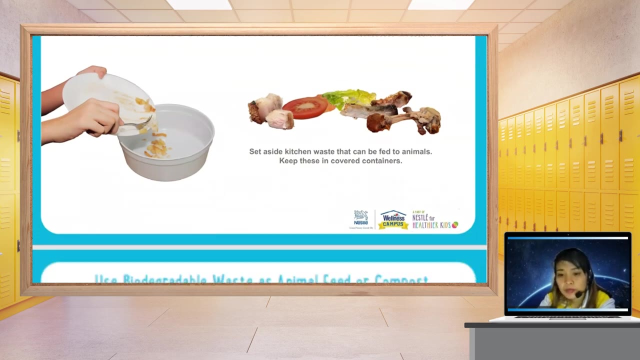 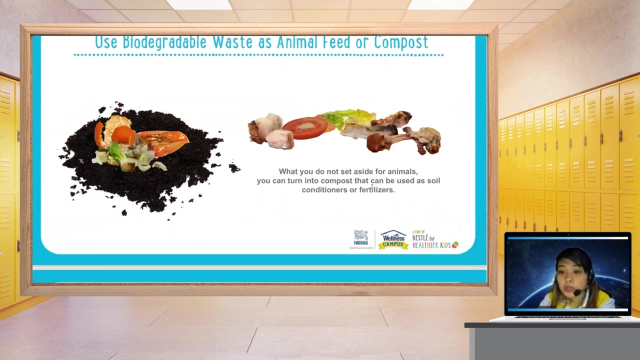 from the trees as well. Okay, so we could use biodegradable waste as animal feed or compost. right, Set aside kitchen waste that can be fed to animals like pigs. keep this in covered containers. Then, what you do not set aside for animals, you can turn into compost that can be used as a soil. 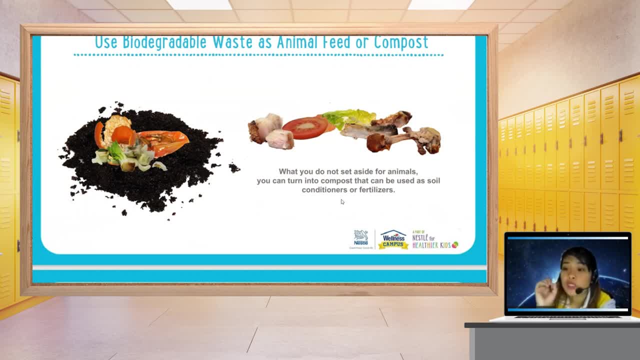 conditioners or fertilizers, because we all know that fertilizers, you know they're not good for the environment, So you know you can use a lot of fertilizers. you know the one that manufactured it can be harmful, right, It can be harmful to us and also to animals, So always separate. 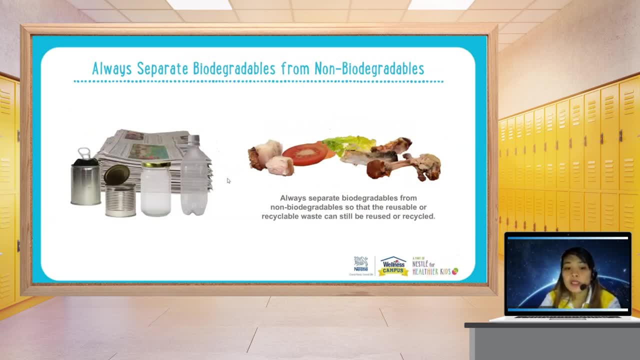 biodegradables from non-biodegradables, right, Just like what we have in the picture. So can somebody tell me what is here in this picture, right? Is this non- or bio? Of course we know the answer right. 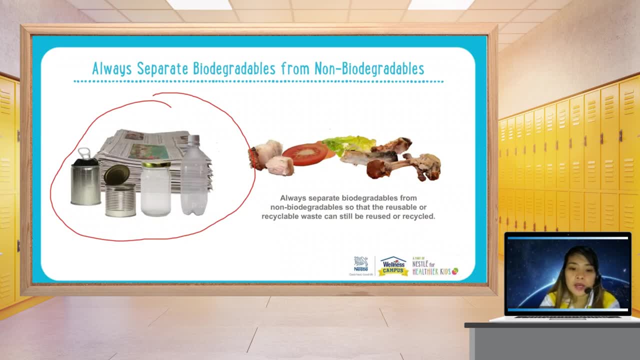 This is the example of non-biodegradables, right, Right. And this one on the other side, right. This picture on the other side: food waste. again. these are examples of biodegradables. okay, Right, So always separate biodegradables. 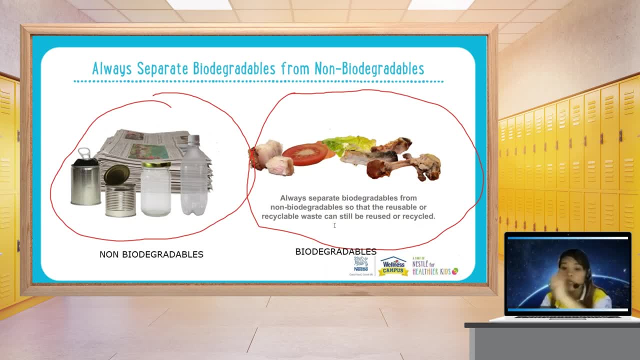 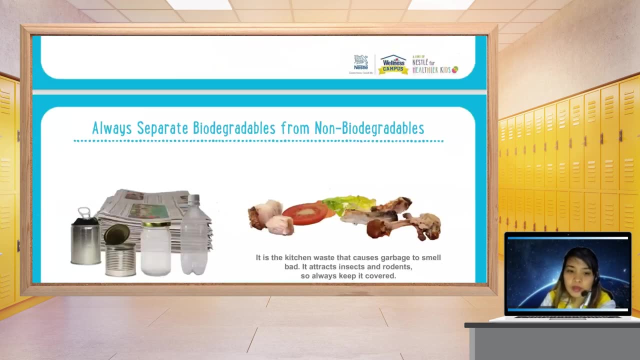 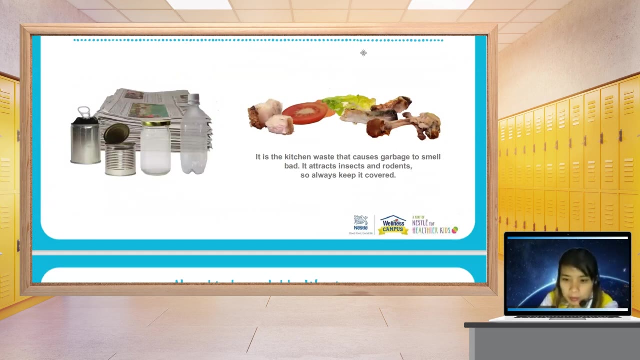 from non-biodegradables, so that the response to the food waste is not harmful. right, So usable or recyclable waste can still be reduced or recycled. all right, Let's move on. So it is the kitchen waste that causes garbage to smell foul, right, Really bad. It attracts. 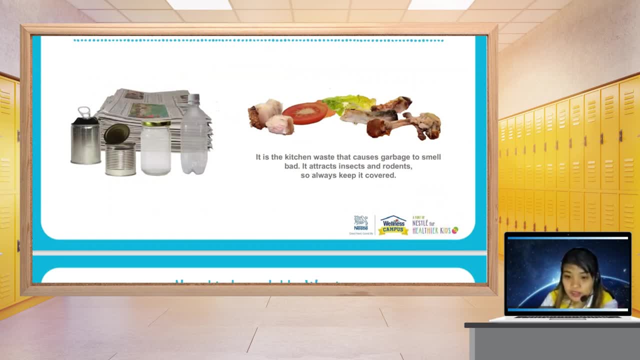 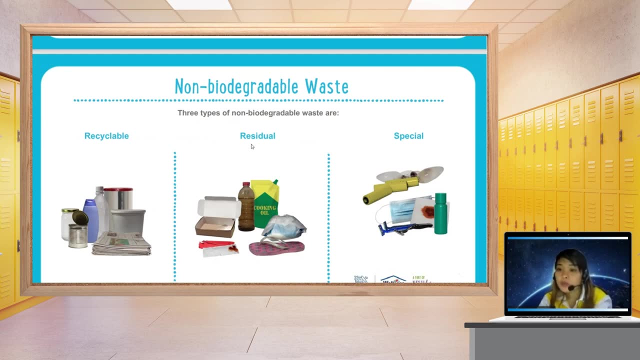 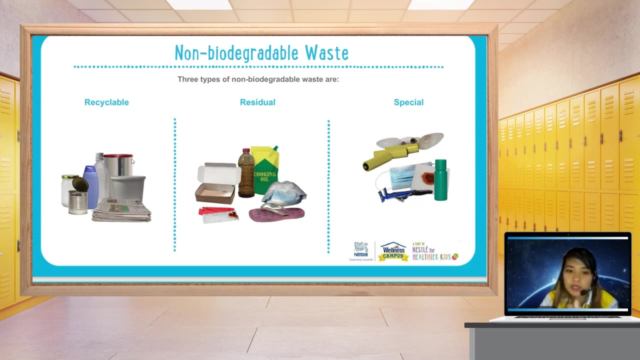 insects and rodents, so always keep it covered. So there are three types of non-biodegradable waste, by the way: The recyclable, the residual, the special right. So, as you can see here an example: recyclable usually, that you can recycle, right, Plastic. 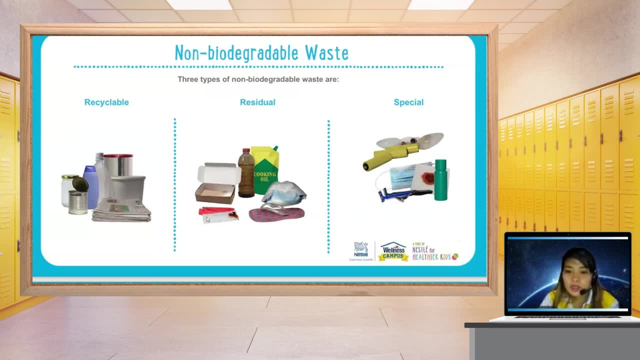 paper cans, residuals, right, You know, when you eat in the fast food, the one, the container, the cooking oil, right, Slippers, diaper, waste, right, Diaper that is used. And these are the special electric electric, you know, old electric fans that cannot be used, something like that. 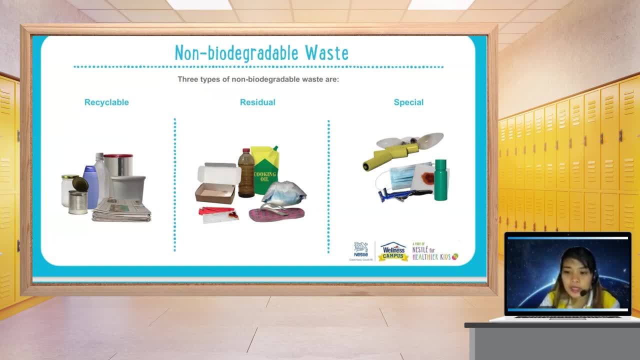 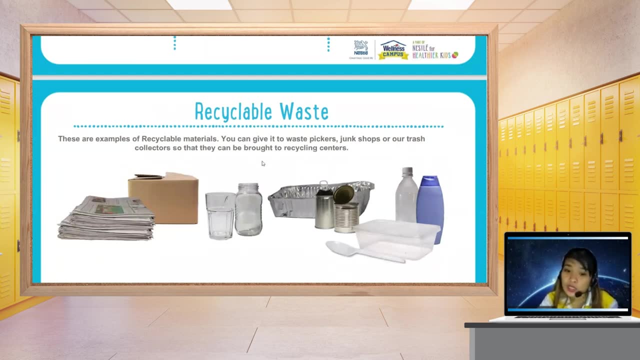 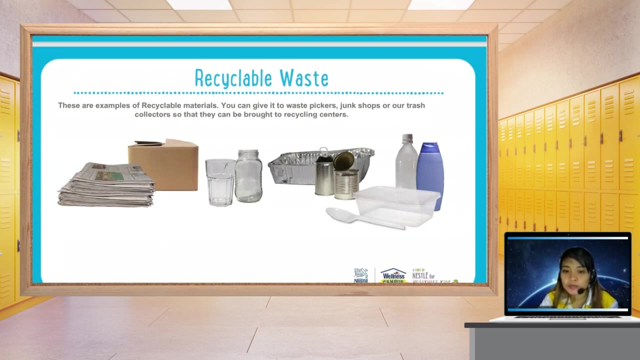 Batteries, masks, gillette, something like that. all right, So these are examples of recyclable materials You can give to waste pickers, junk shops or trash collectors. right So, because they could put them into good use. right The plastic bottle, the paper. right The can plastic container. 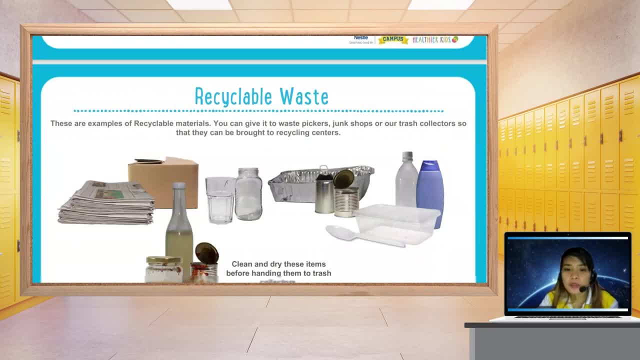 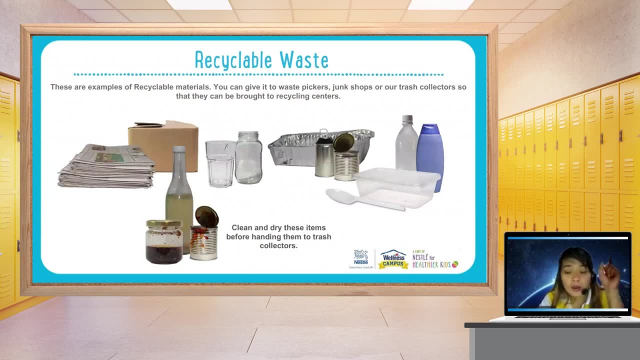 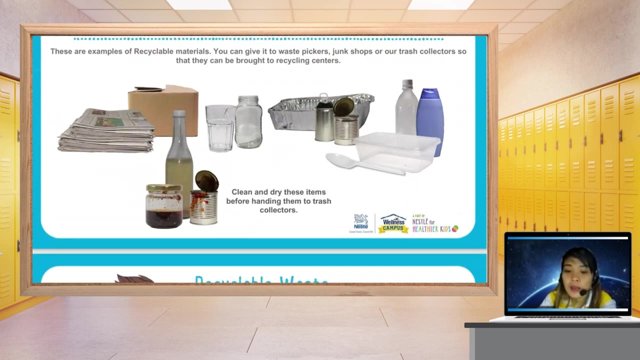 they can use that again, And these are examples of recyclable materials You can actually give away, just like what I've been mentioning earlier, But before you give them out, you should clean and dry these items before handing them to the trash collectors. okay, And what about? 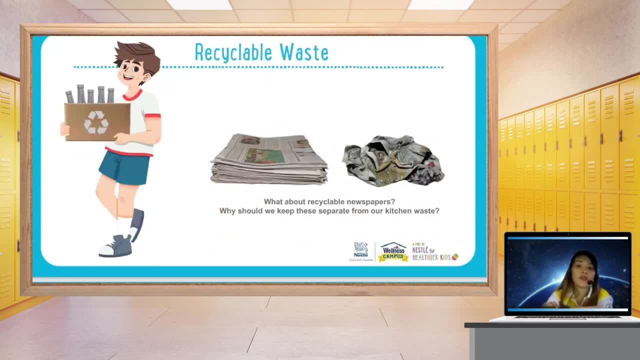 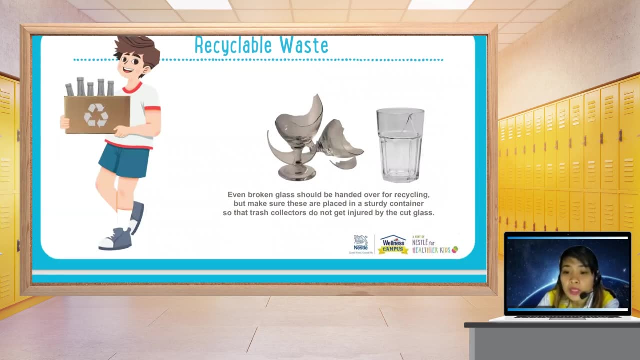 recyclable newspapers. What do we do with them, dear students? right, Why should we keep these separates from our kitchen waste? Even broken glass should be handed over for recycling. okay, But make sure these are placed in a sturdy container so that it can be used for recycling. 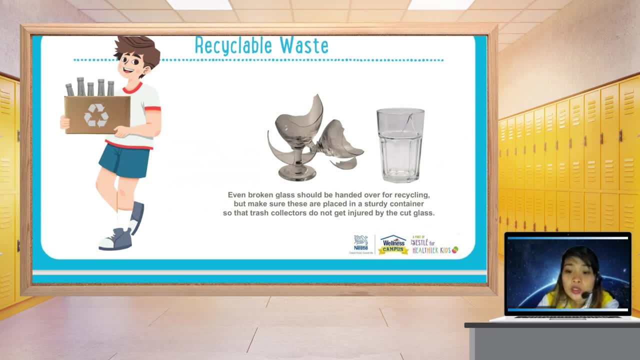 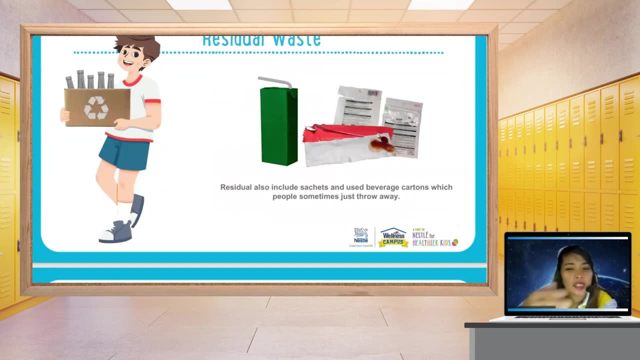 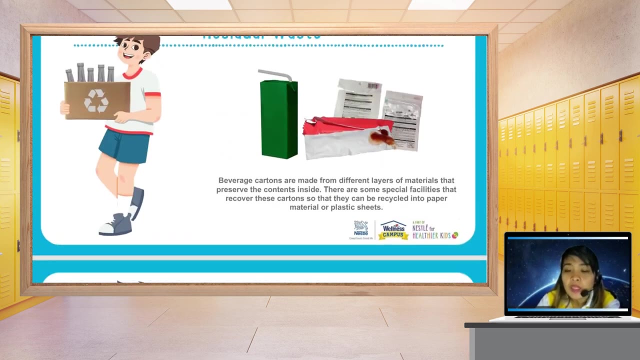 So that's why we have these And the trash collectors will not get injured by the cut glass, And recyclable also includes sachets and use beverage cartons, which people sometimes use throw away. Beverage cartons are made from different layers of materials that preserve. 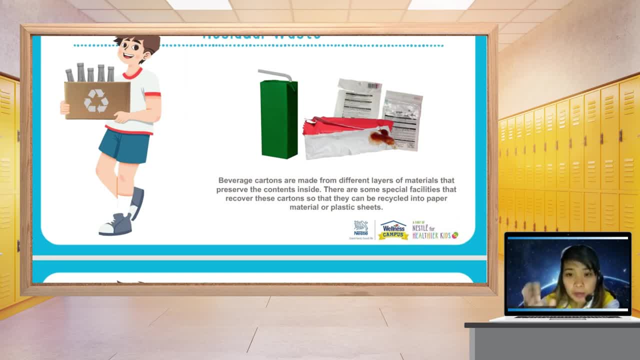 the contents inside right, Like the milk, for example. There are some special facilities that recover these cartons, and they're actually thrown away by trash collectors so that they can be recycle into paper material or plastic sheets. Sachets can also be collected for alternative recycling. 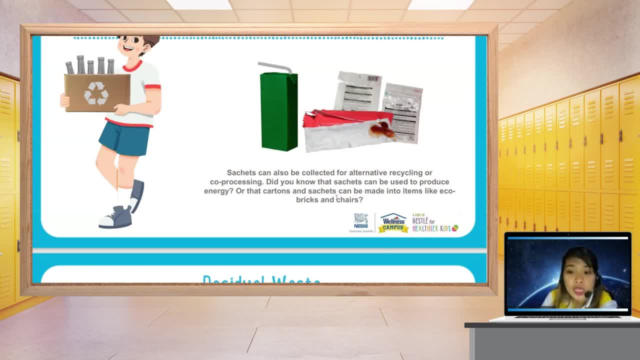 or co-processing. So did you know? there are students that sachets can be used to produce energy, right. Or that cartons and sachets can be made into items like eco-bricks and chairs, right. Okay, So we have. 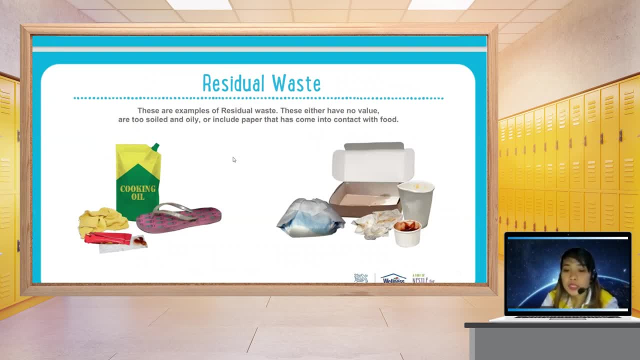 here some examples of residual waste. So these are examples of residual waste. These either have low value, are too soiled and oily, or include paper that has some contact with food- right, Like cooking oil. right, Diaper that has poop on it, right Okay. 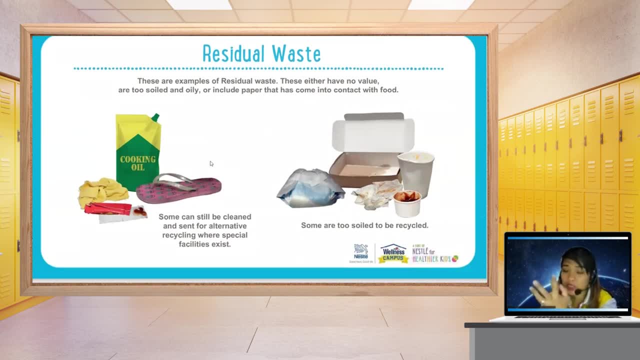 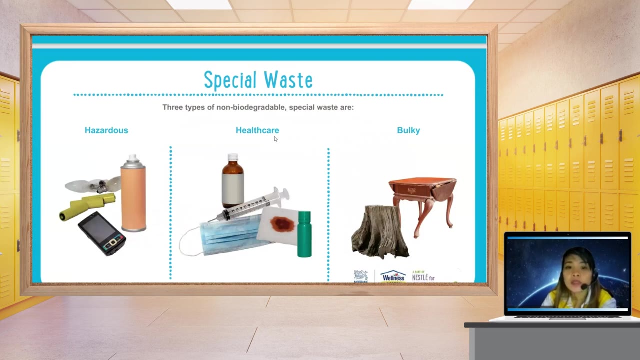 And some can still be cleaned. right, We can still actually clean them for alternative recycling where special facilities exist, but some are too soiled to be recycled. So what about special waste? These types of non-biodegradable special waste are hazardous, right Healthcare. 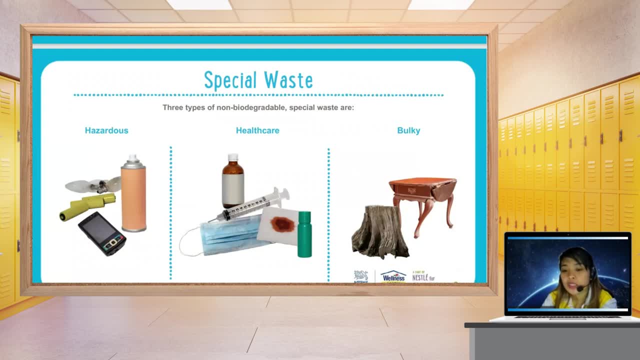 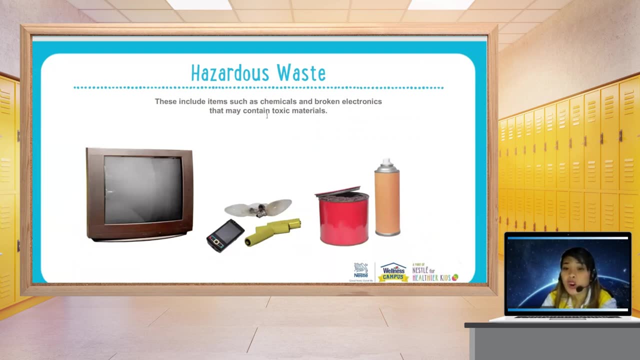 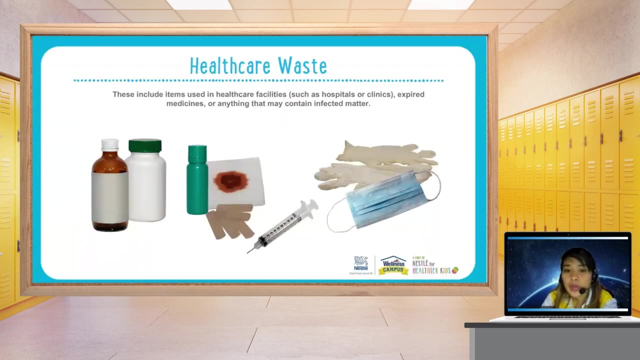 bulky right, Old chairs tables right And hazardous. waste does include items such as chemicals and broken electronics that may contain toxic materials, especially batteries right, They're not good for the health And healthcare. waste, of course, does include 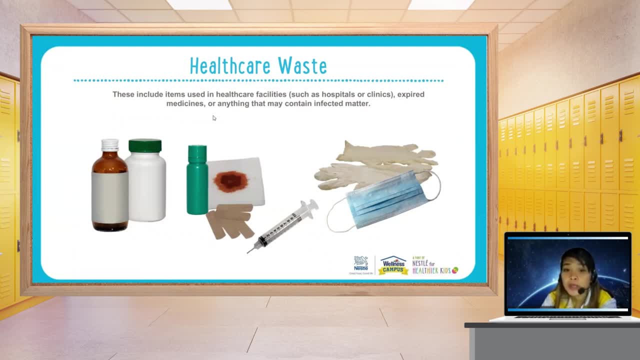 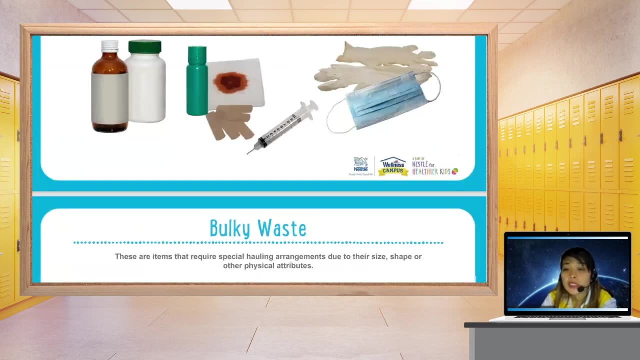 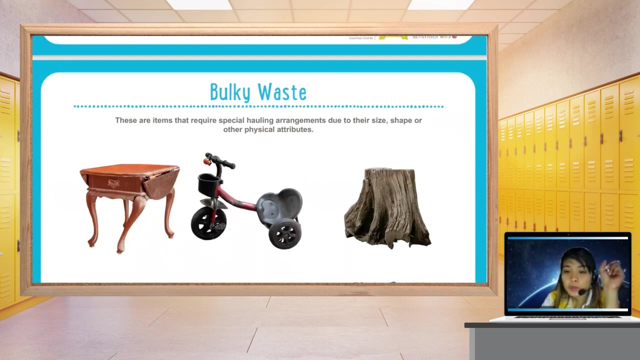 items in healthcare facilities, Such as hospital or clinics, expired medicines or anything that may contain infected matter, especially now, right That we still have COVID-19. So you know we must therefore dispose them properly. Bulk waste requires special hauling arrangements due to. 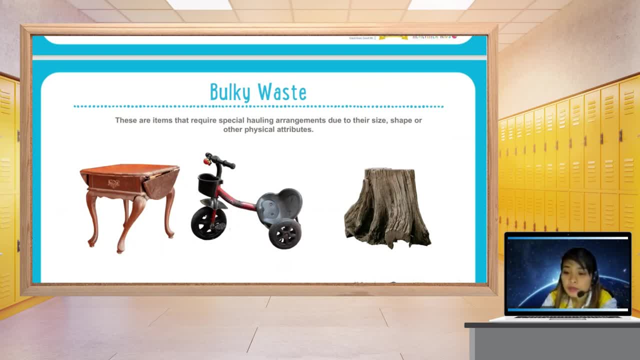 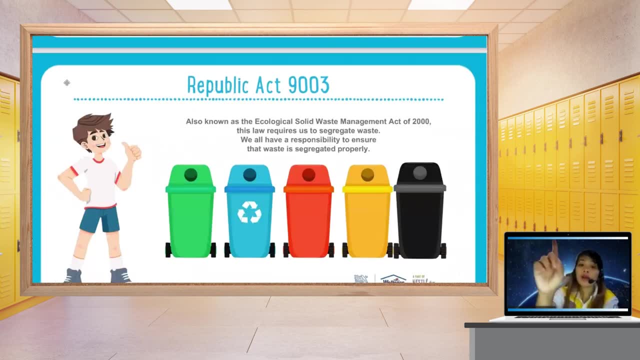 their size, like an old bicycle, an old table, right? So do you know, if you're a student you've gotta pick up all the serious stuff first and make sure you take care of all the things in it. So then we get back to the 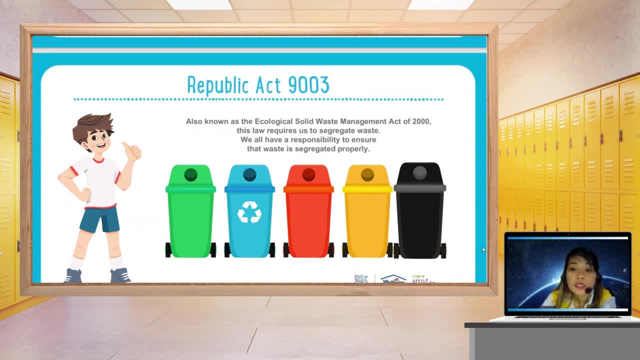 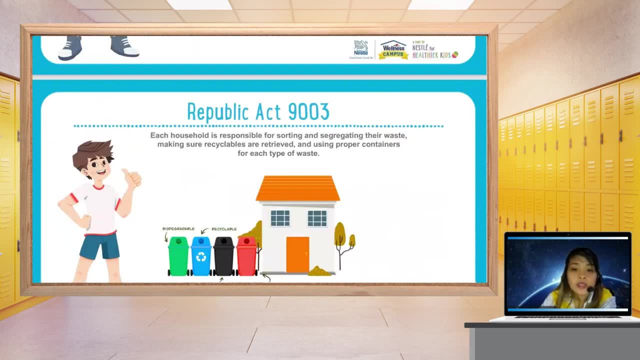 map again is that we have like Republic Act 9003, also known as the Ecological Solid Waste Management Act of 2000.. So this law requires us right Citizens to segregate waste. We all have our responsibility to ensure that waste is segregated properly. So, as you, 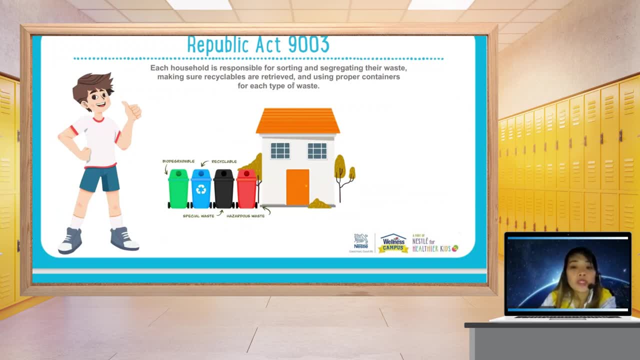 can see we have eight different colors of trash bins right, So each household is responsible for sorting and segregating their waste. Make sure recyclables are retrieved and using proper containers for each type of waste. So, for example, the green one is for the biodegradable. 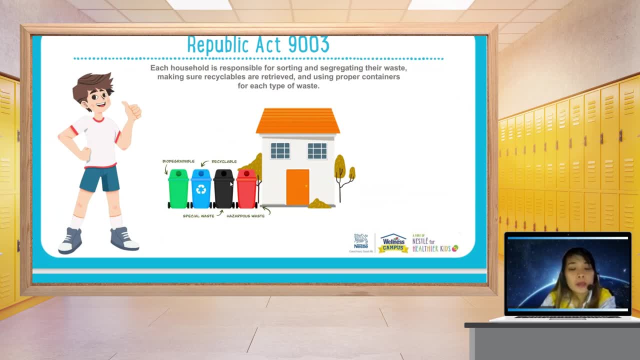 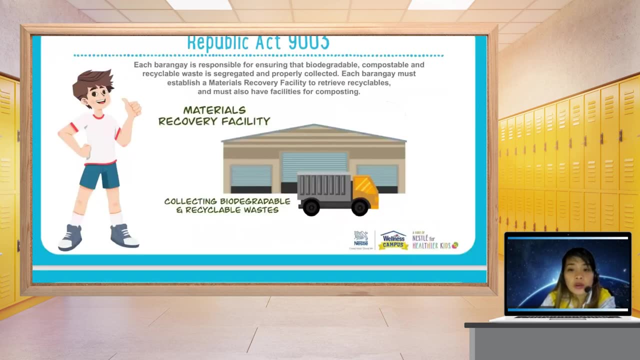 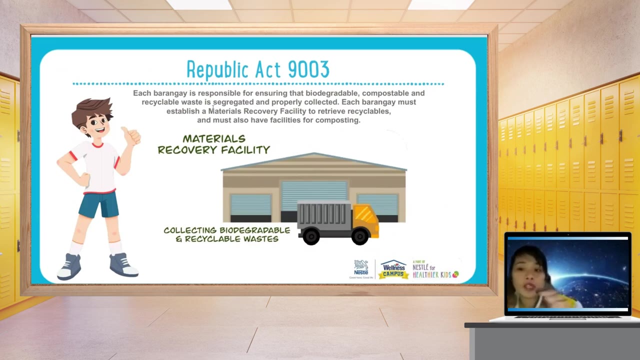 The blue one is for recyclable, The black one is for special waste And the third one is for the hazardous waste. All right, So Republic Act of 9003 also states: each Burmese guy is responsible for ensuring that biodegradable. 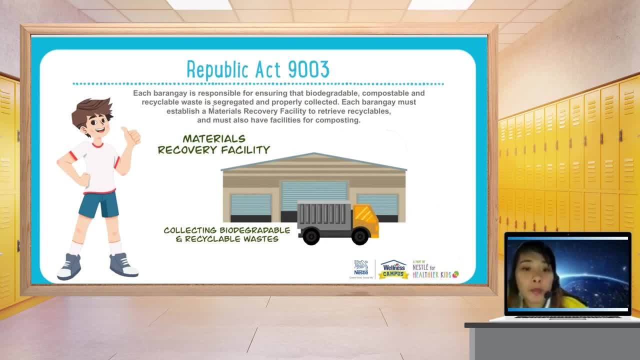 compostable and recyclable waste is segregated and properly collected. Each Burmese guy must establish a materials recovery facility to retrieve recyclables and must also have facilities for composting materials. So, as we can see here, we have a materials recovery facility. 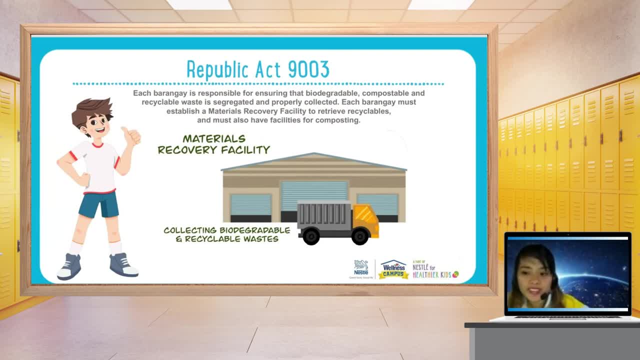 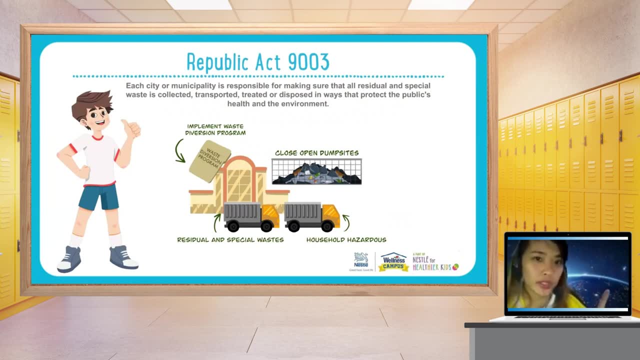 collecting biodegradables or recyclable waste. Okay, All right. So also in Republic Act of 9003, each city- just like here we have, we are living in Captain City- each city or municipality is responsible for making sure that all residual 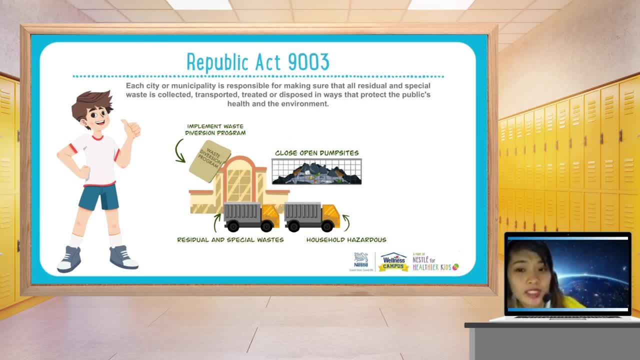 and special waste is collected or transported, treated or disposed in ways that protect the public's health and the environment. Right, Just like we have here closed open dump sites, Right So it's segregated: the residual and special waste and the household hazardous. 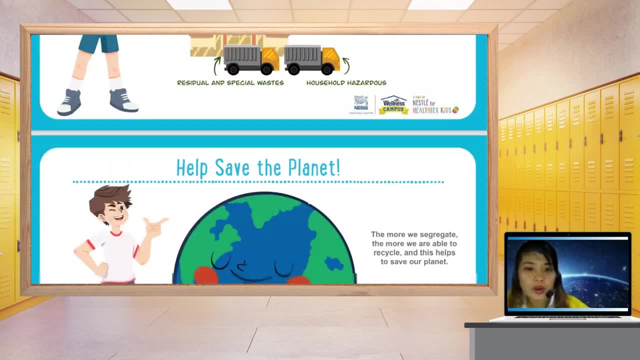 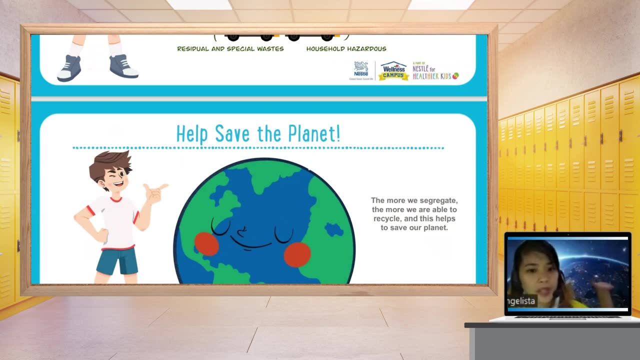 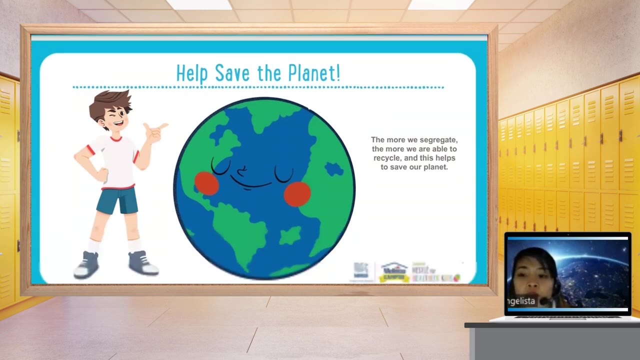 Right, Okay, All right. So we should help save our environment. All right, Right, Help save the planet, just like what we have here. So the more we segregate, the more we are able to recycle, and this helps our environment.